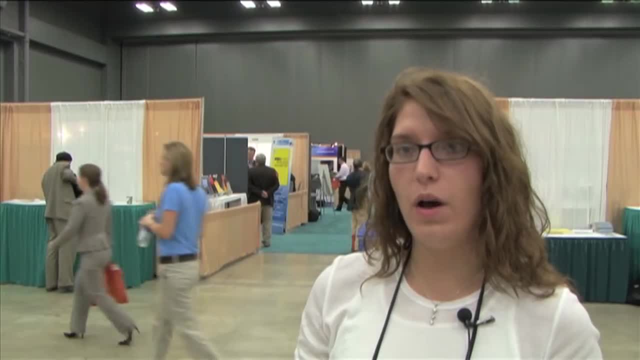 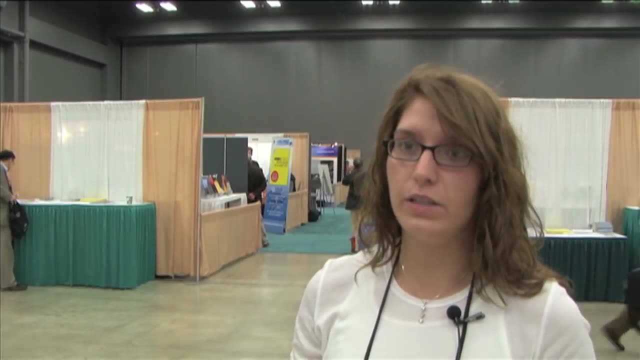 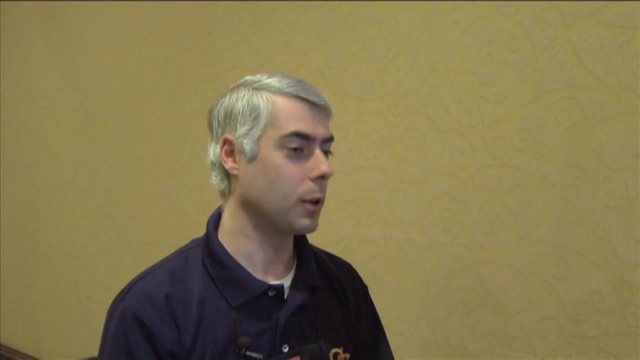 electricity and then we're going to put that into a simulation model and simulate that this event could happen a thousand times and output results that the simulation tool gives you an advanced look at something that you can't collect data over time for One of the more fun things that I do is NCAA tournament predictive models. We use some 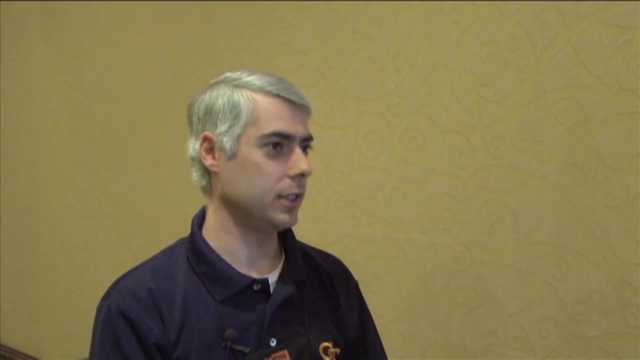 Bayesian probabilities, some Markov chain models, some logistic regression and have a pretty good predictive model of which teams will do well in the NCAA tournament, which teams will go further. And so I guess three years ago now we predicted the whole last three rounds correctly before. 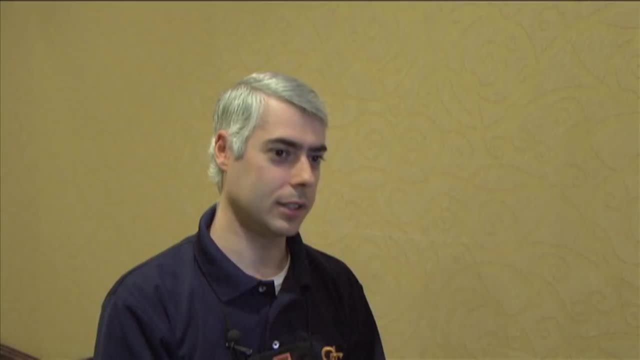 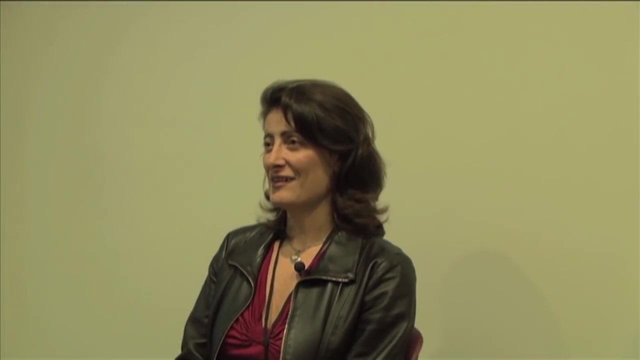 the tournament even started Last year. there was a website that tracks 50 or so different predictions, and our method beat the other 50 by at least three games, So that's a fun project. Supply chain optimization basically involved trying to predict what's going to happen in. 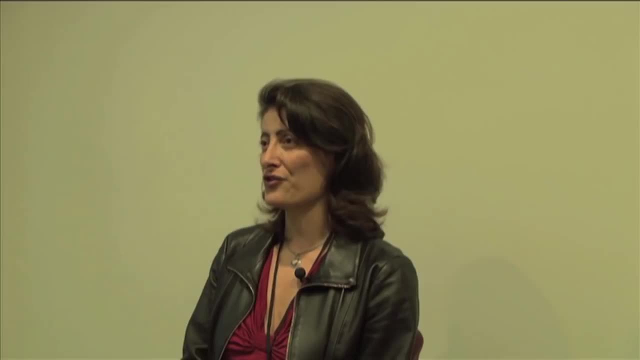 the future, And so the goal is to understand how to make the best decisions in order to acquire the materials that you need in order to manufacture products or to assemble different products. So, for example, if you are building a laptop computer, clearly there are a lot of different. 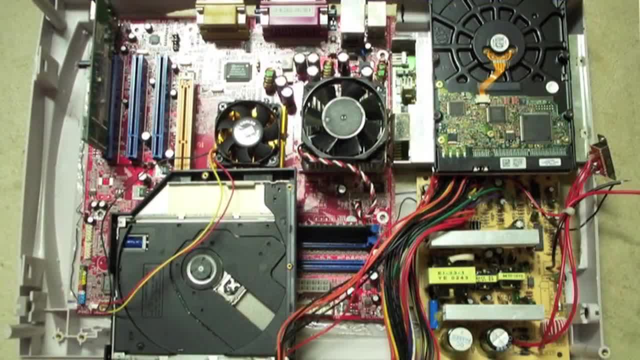 types of components that go into that, and companies such as HP and Dell, et cetera have to make decisions about how many of each different type of component to manufacture. And so we're not just going to ask you to build a laptop computer, we're going to ask: purchase? When should they purchase them? In what quantities should they purchase them in order to take advantage of different sorts of economies of scale? So supply chain optimization involves basically trying to figure out what to buy, when to buy it and at what price. 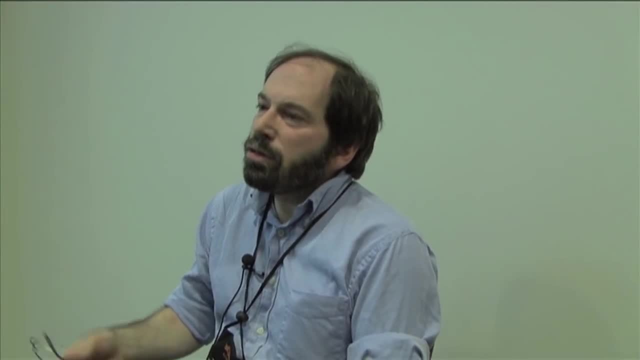 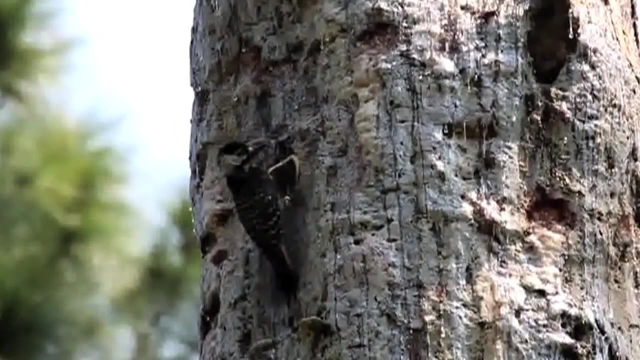 But, on the other hand, I've been working on a problem or a set of issues which we like to call computational sustainability. So I've been working on trying to save a species of woodpecker that, if this is the red cockaded woodpecker, it's on the endangered species list, And so we're. 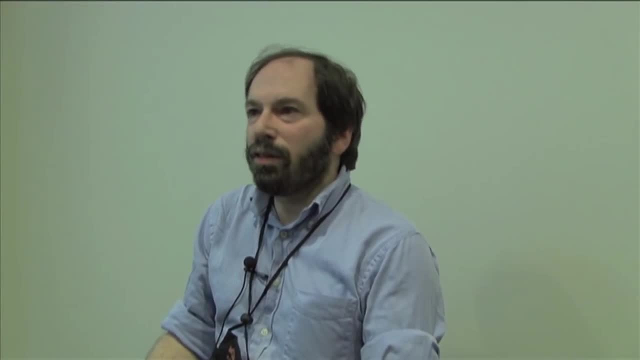 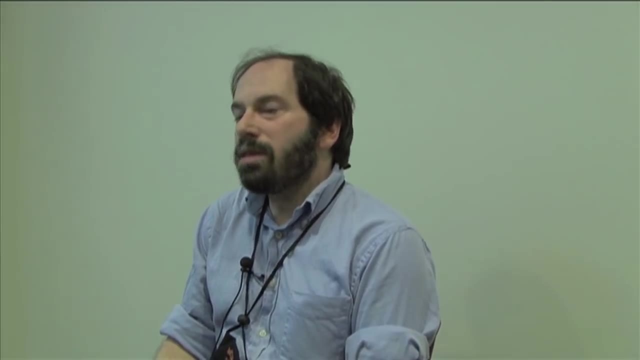 trying to understand how we can guide again, give quantitative models for thinking about how to allocate funds so that the conservation fund, which buys tracts of lands for the preservations of species, So this is, you know, entirely different range things, The same sorts. 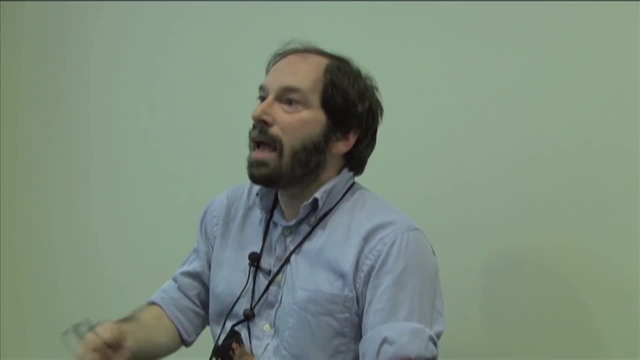 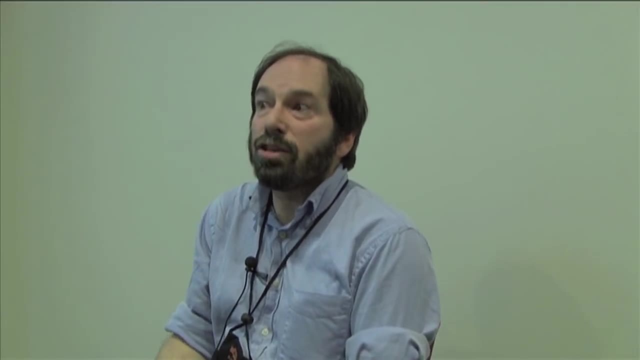 of issues come into play. You've got degrees of stochasticity, their randomness, and how the birds populate, how things affect them, But you've got limited resources, the money in which to spend, in which to make the system as efficient as possible. Okay, so, in particular for the 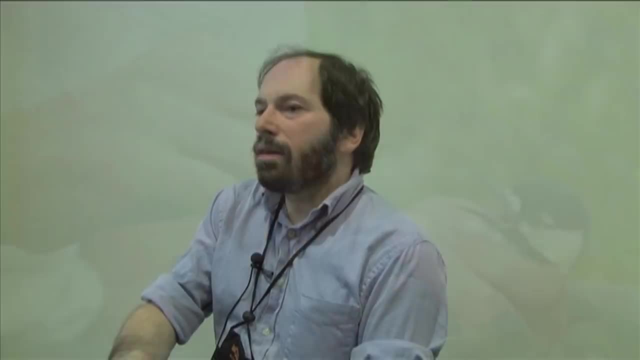 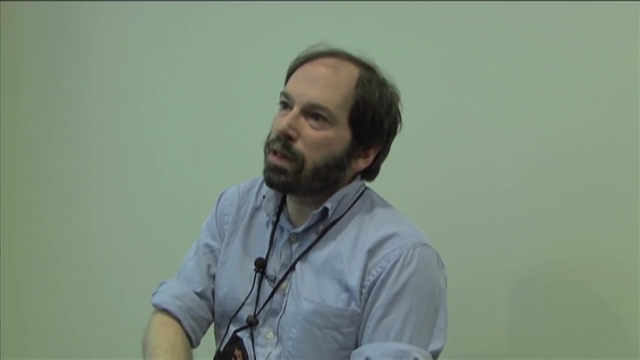 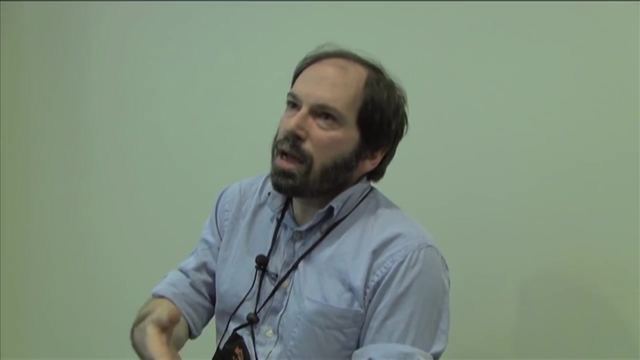 woodpecker project. it really boils down to a very large scale. first, initially stochastic integer program, but in fact we're solving with, then simulating it through a deterministic integer program. The range of land means that we're solving a network design problem on millions. 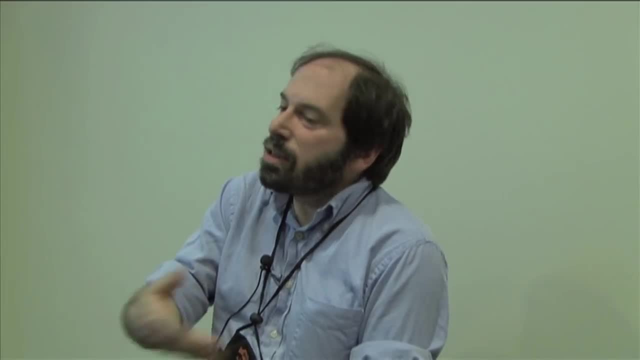 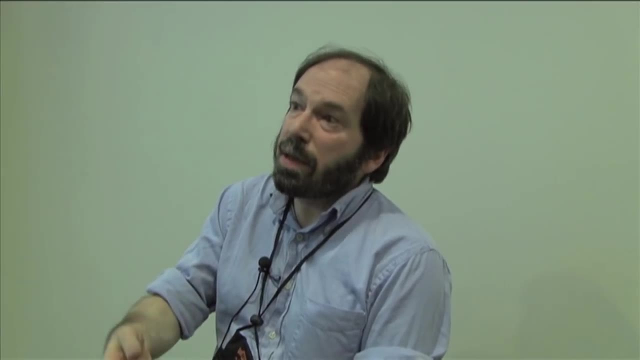 of nodes. And you know, twenty years ago this wouldn't have been thought and it hasn't. And it's not just the advances in computers. of course that's an important role in terms of the availability of large-scale memory and the like, but it's really the advances. 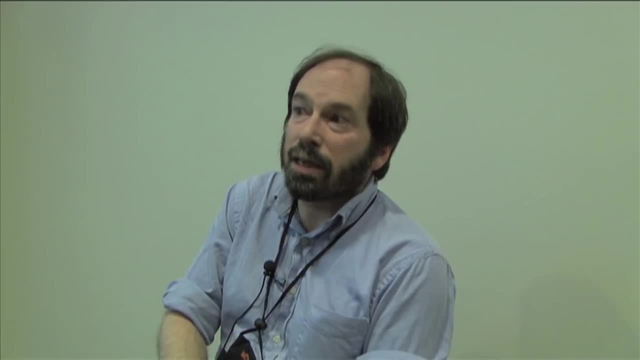 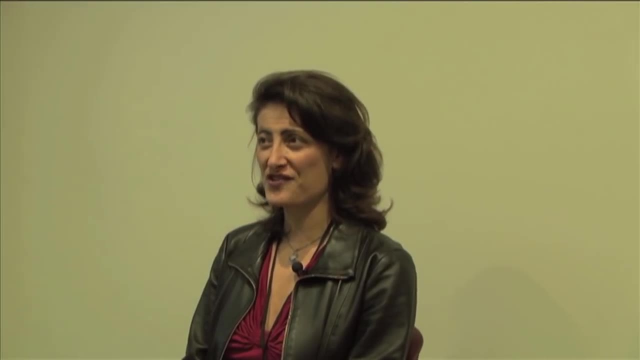 in methods to attack these problems. that has really been the driving force of why we can actually get reasonable solutions. So I've worked on a number of different projects over the course of my career, both in academia and outside of academia. One that particularly comes to mind was a project that I worked on several years back. 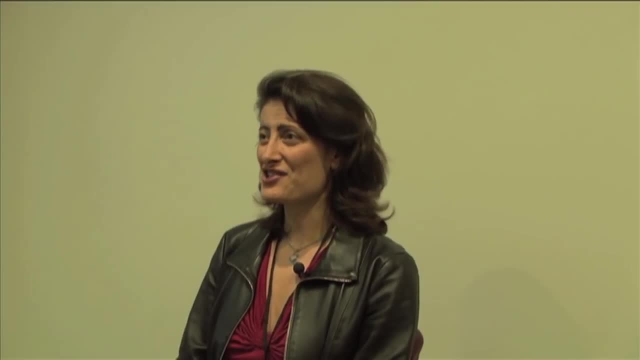 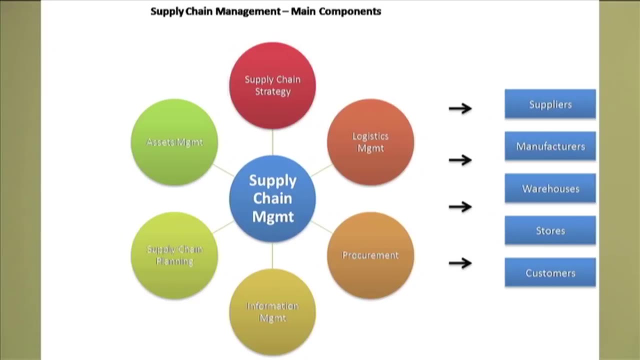 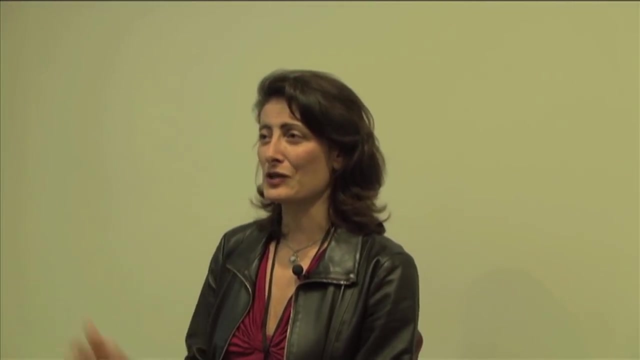 while I was working for a company as a supply chain optimization consultant And we worked for a plastics manufacturer, so a manufacturer of injection molded plastics, all the kinds of things that you can go out and buy it choose your biggest, your favorite big box store and you need to move and you go out and you buy a lot of plastic tubs with. 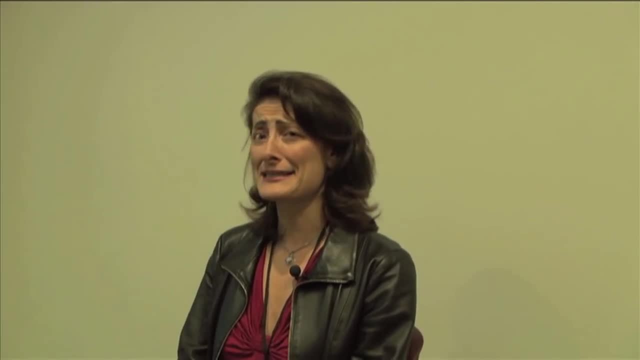 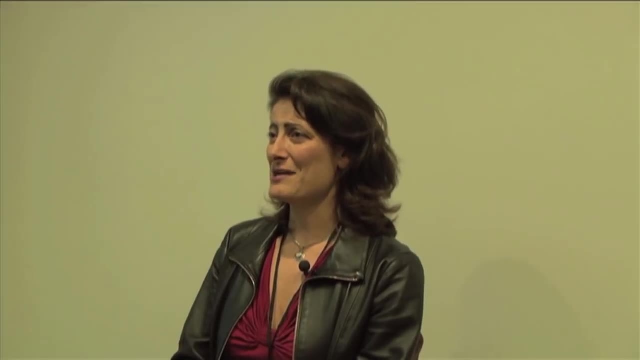 tops or different laundry baskets and things like this. So this is basically a company that had a very interesting manufacturing environment. Lots of different types of molds that were in place. these are basically- you can think of them as the shells that hot plastic gets squirted into and then, several seconds later, 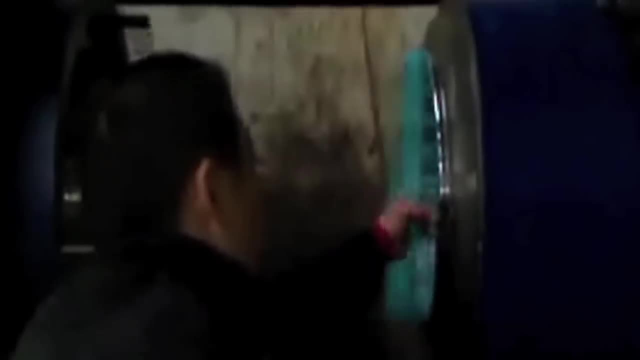 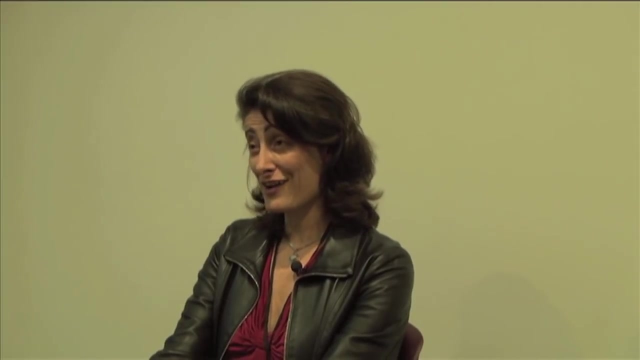 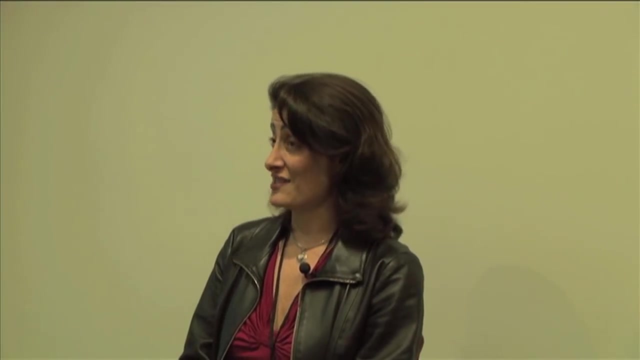 mold opens up and out pops a purple laundry basket or a purple tub or something like this. So one project we were involved in was to helping this particular company schedule their manufacturing operations And it was very interesting. It was very interesting because it involved a lot of different sorts of discrete optimization. 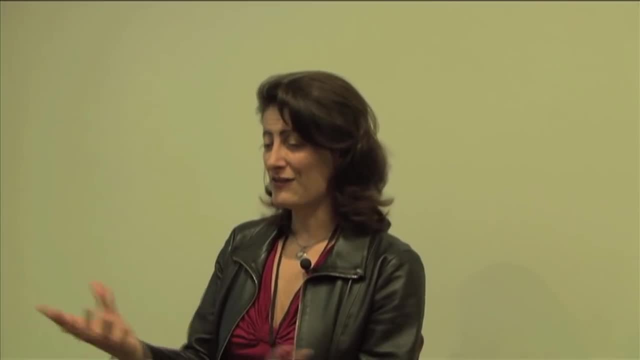 problems You wanted to figure out, not only, given you have a certain number of machines, what sorts of tooling you wanted on those machines- think of it as what sorts of shells you wanted to put on there- but also there then came the question of: okay, so if I have the tool that 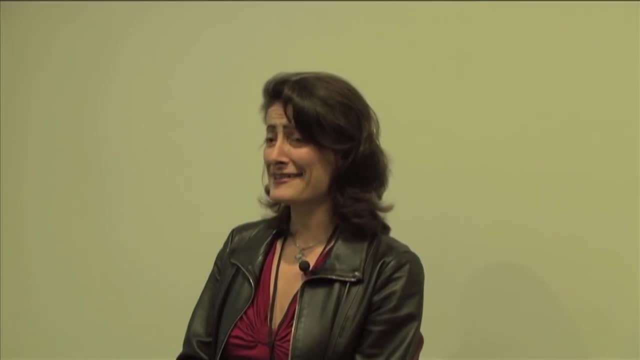 is a laundry basket. okay, now I'm going to make a lot of different colors of laundry baskets, And what order am I going to make those? Clearly, it wouldn't make sense to make white laundry baskets and then immediately switch over to black or very dark laundry baskets. 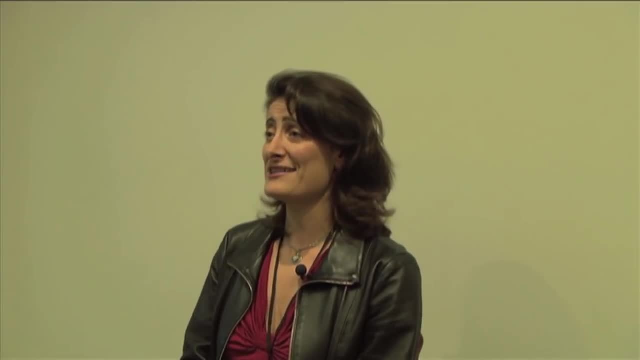 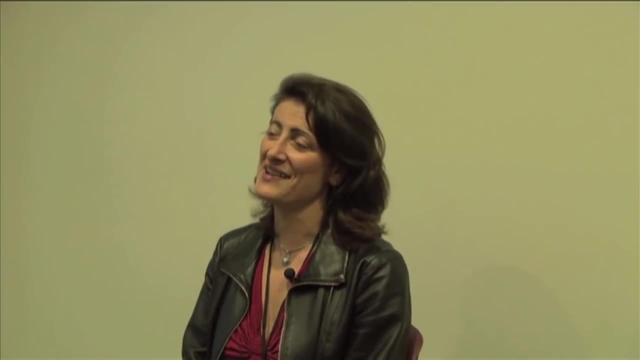 So there were all kinds of interesting scheduling problems where we had to think about not only what sorts of products to make, when, how many of those products to make, but also a color sequencing aspect of it, And that was really a pretty interesting problem that clearly involved a lot of OR types of 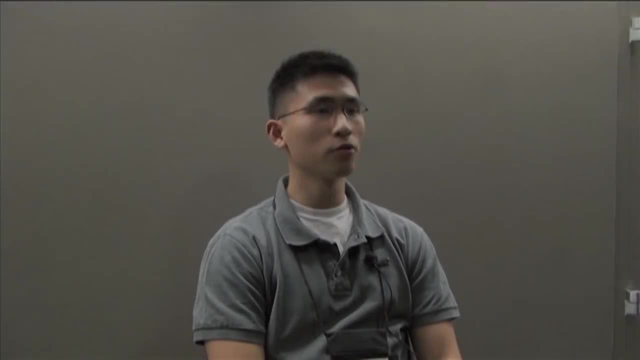 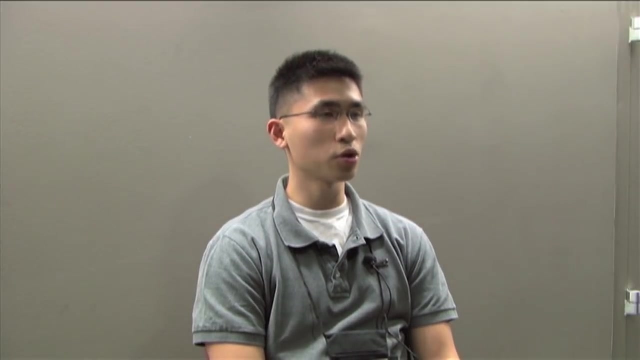 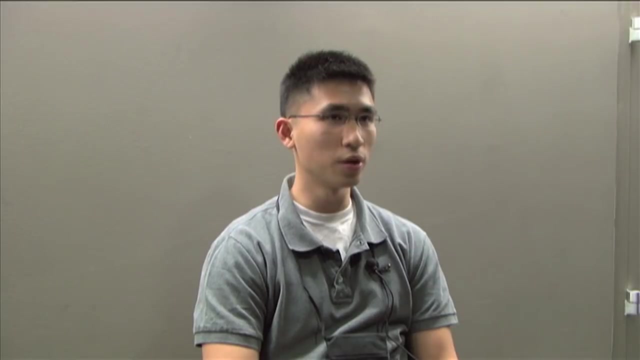 modeling as well as solution approaches to solve. Yeah Yeah, One of my thesis was stochastic terrain profile modeling And I'm trying to use that and relate it to operations research. It also had to do. I mean, I guess, if you would extend the research, it also had to. 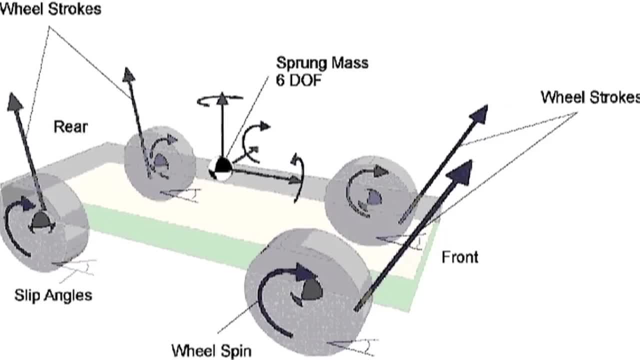 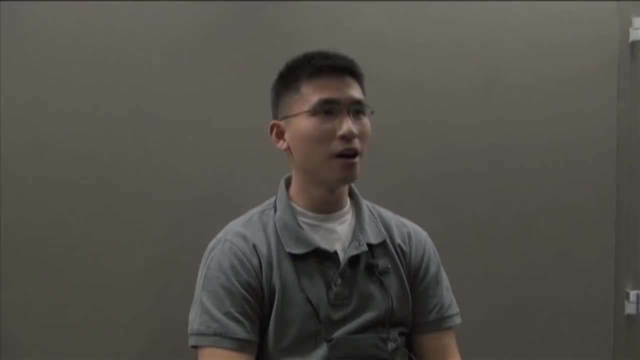 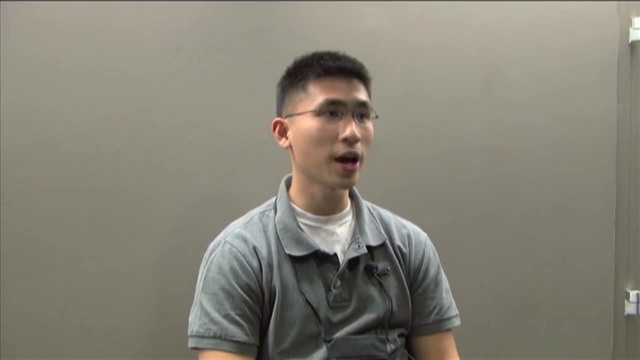 deal with field efficiencies more of a vehicle dynamics aspects, So it relates- I think it relates- to ORs in several aspects of that nature. The concept of that is to create the topology of the terrain. I'm also incorporating stochastic soil models. 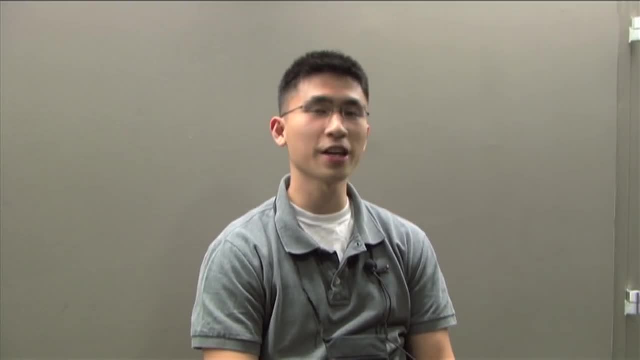 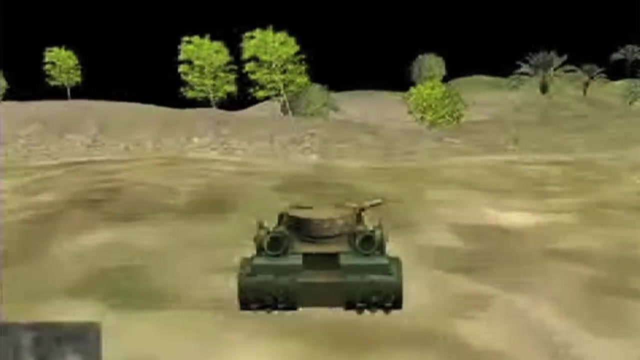 But I guess taking a step back- I mean I think that's very detailed, taking a step back and understanding what that is. It's more for vehicle dynamics understanding. let's say, for example, for the Army: you want to send a tank over to Iraq. 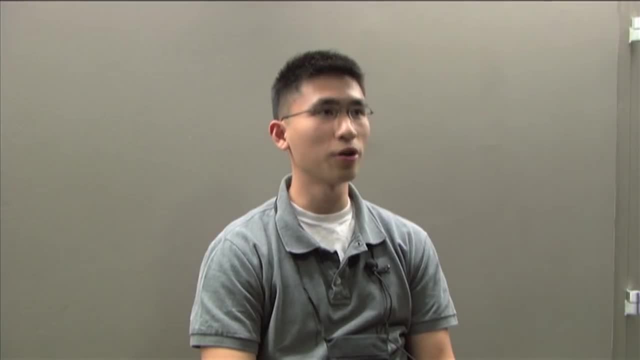 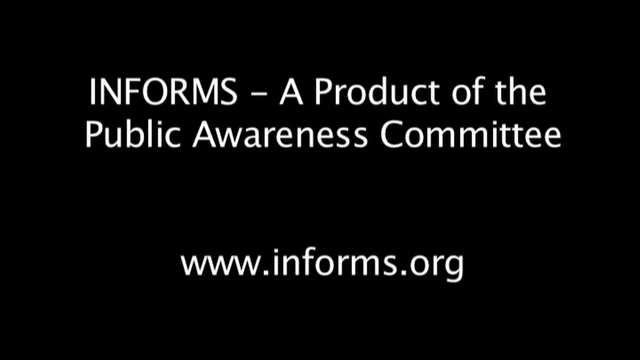 You have to create your vehicle, create your suspension so it could fit your terrain models, And you have to, of course, have a lot of data and information to help you see where they are in the environment. But in the course of a lot of that, you have to do a lot of research. And so you know, in the course of a lot of those tests- a lot of it is you know- you can just start with a little bit of information and you can do a lot of sitting in the park with it, And that's what I was looking for. I was looking for the tool. I was looking for the location. 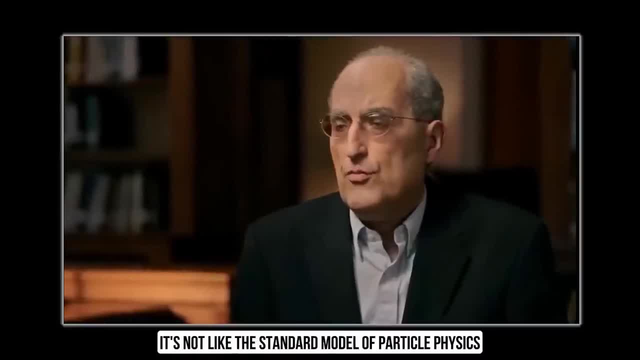 String theory is certainly not a well-established theory. It's not like the standard model of particle physics or like Einstein's theory of gravity. We've come a long way since Einstein's alleged refusal to accept a universe ruled by the rolls of the quantum dice. Schrödinger's